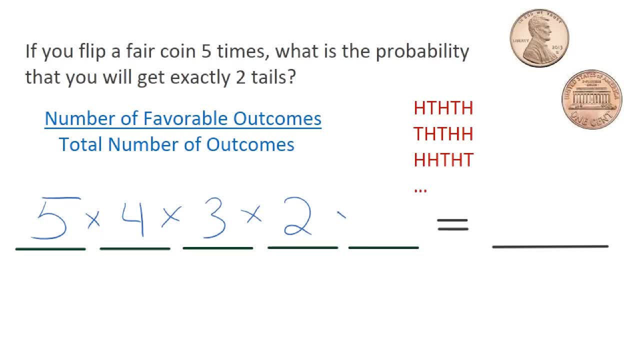 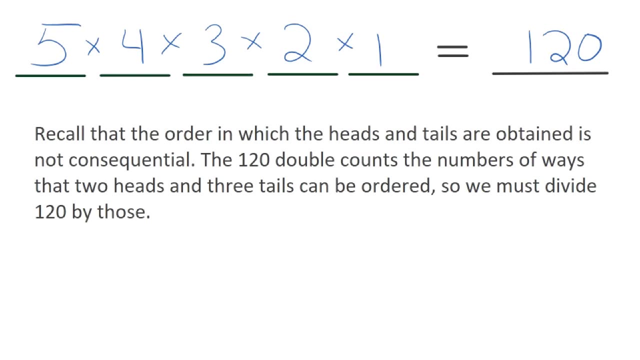 and then three, then, of course, two and one. So this is the same as five factorial, or five times four times three times two times one, and that is one hundred and twenty. What we must consider, though, is that this value one hundred and twenty. 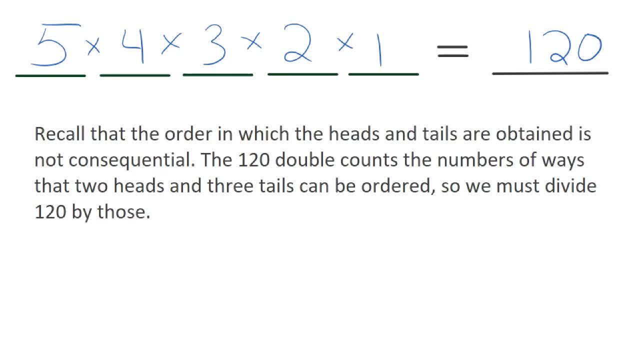 is double counting the number of ways that two heads and three tails could be ordered, And remember, order doesn't matter. So we need to make sure we don't double count those iterations, and so we have to divide one hundred and twenty by those. 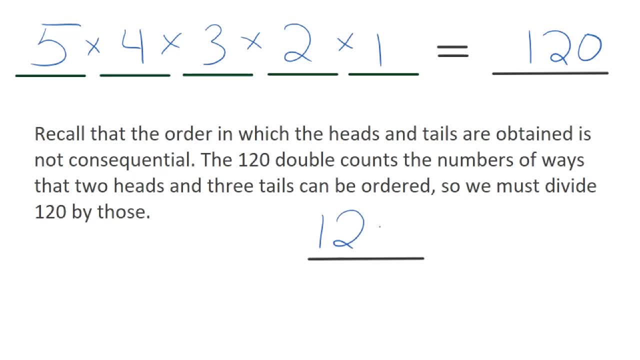 So that will be one hundred and twenty divided by the total number of ways that we can arrange two items and the total number of ways that we can arrange three items, And so this becomes one hundred and twenty divided by two. factorial is just two. 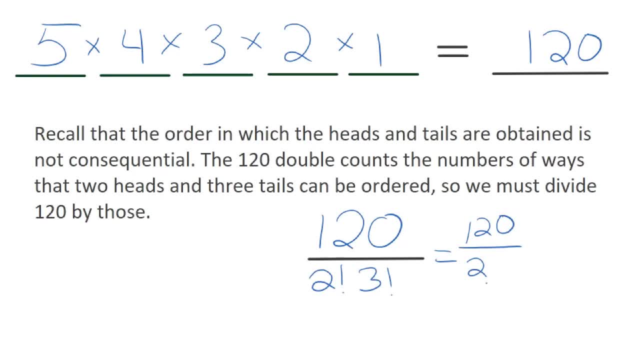 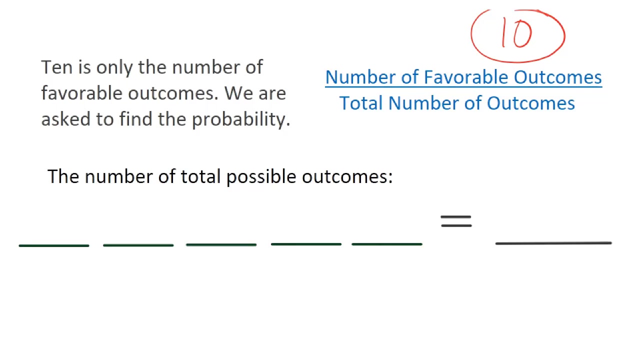 three factorial would be three times two times two times one, so six, and this equals one hundred and twenty divided by twelve or ten. Ten is only the number of favorable outcomes, but remember, we're asked to find probability. so in addition to the number of favorable outcomes, 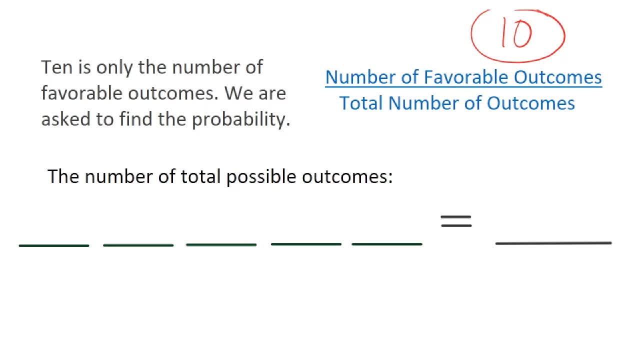 we need to find the total number of outcomes, even those that we would consider unfavorable. in this example, Consider the first flip of a coin. Well, there are two possible outcomes: a head or a tail. and we're neglecting for a moment this bag that we had earlier of five letters. 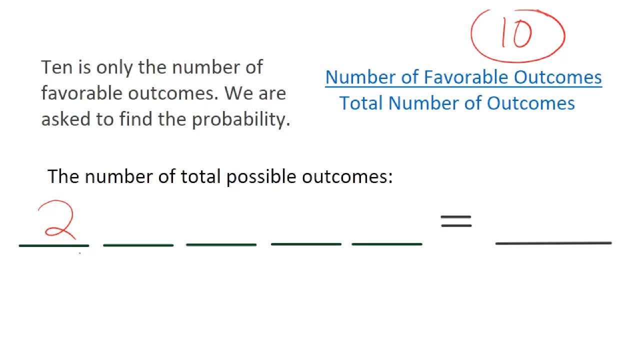 H's and T's, three H's, two T's, and now we're just considering a general coin flip, Two options: a head or a tail on the first flip, a head or a tail on the second, and so on. 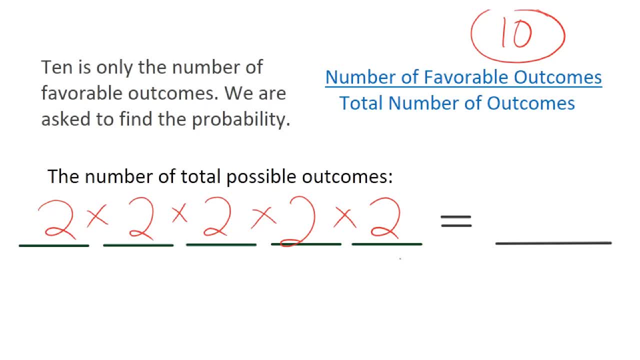 And that of course equals two to the one. two, three, four. fifth power, and that is thirty-two. So continuing, we'll write our probability as the number of favorable outcomes ten divided by the total possible outcomes thirty-two.